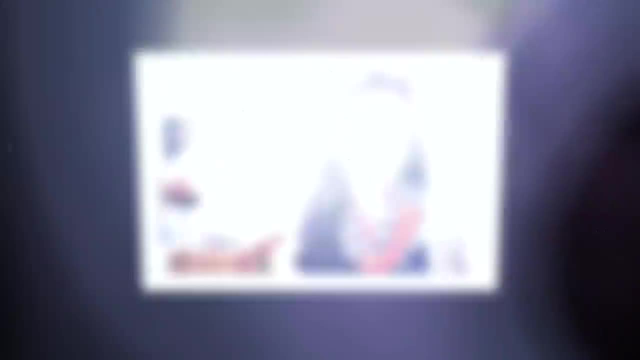 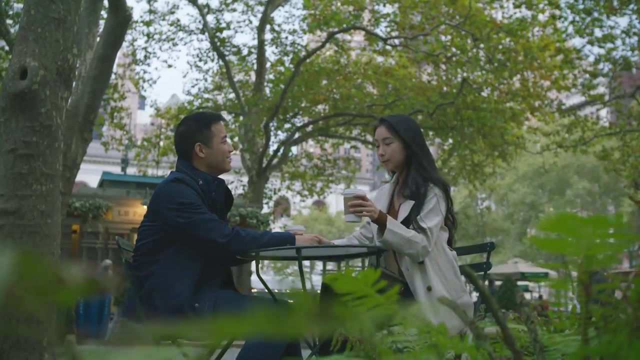 new to the United States. They're not In those videos we see online. someone always has to tell some Asian person or other race to go back to their own country. Most of the time, the person they're talking to is from the country. Asians make up 9% of the nation's overall population. 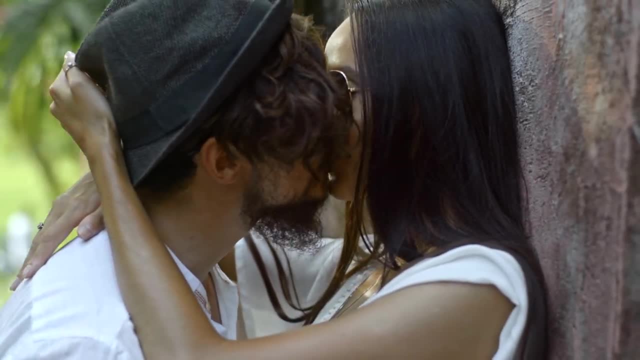 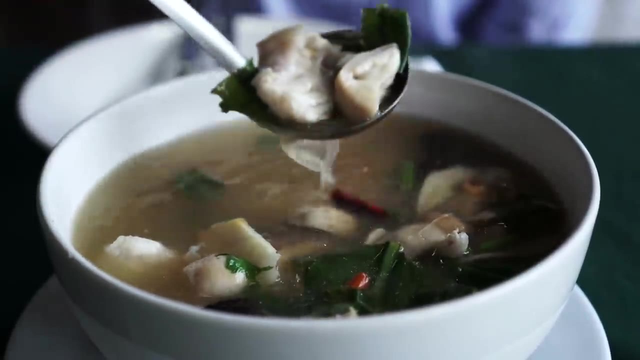 and that's up from 5% in 2010.. So if you think Asians aren't Americans, you're wrong. Today we're just looking at the states with the most Asian residents. Now, this could be good for a lot of different reasons. One: it kind of shows you that Asians 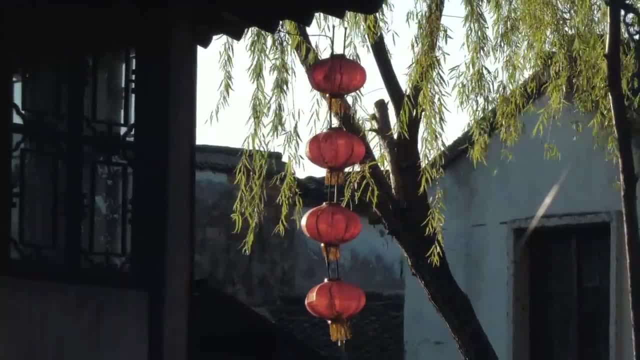 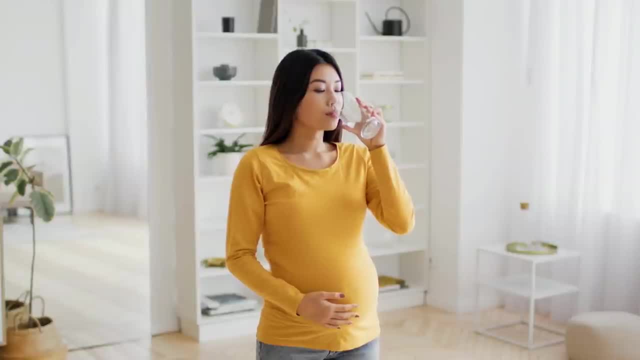 are everywhere here in the United States and they are just as American as anyone else. Also, I get a lot of requests from people from different countries wanting to know where maybe certain populations are, certain races, certain cultures. They want to know where they could find the highest. 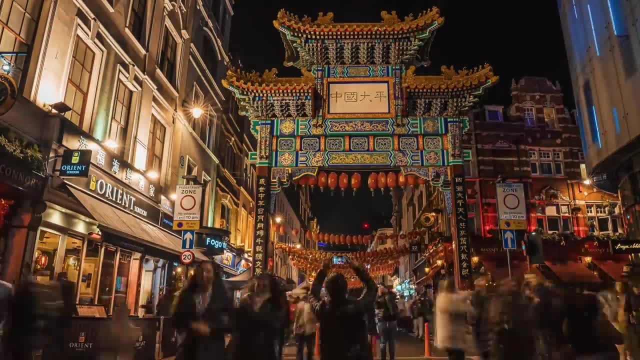 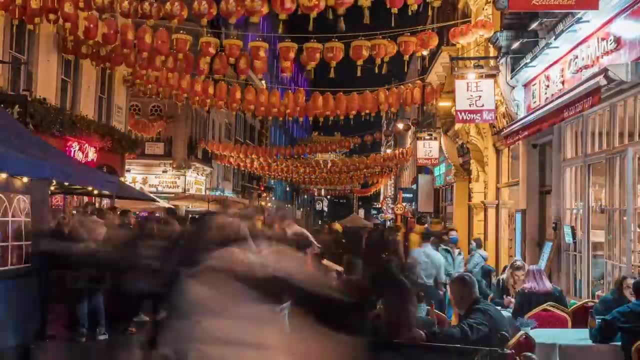 population of people similar to them. That's fine. Now, for reference, Texas is considered to have the average amount, which is 5.2% of their population is Asian. That's according to the US Census. That's how it's being ranked by the states with the highest percentage of their population being 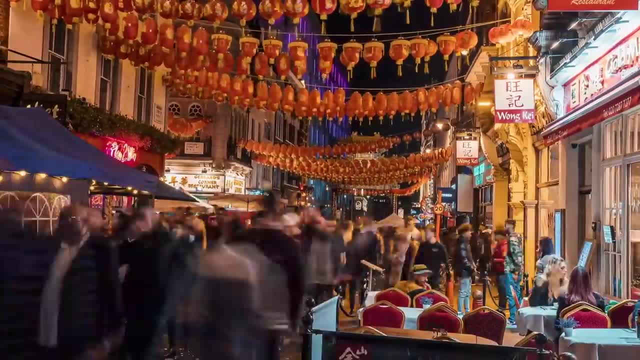 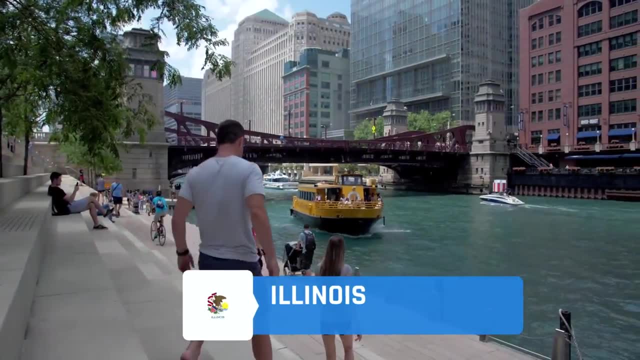 Asian. We'll also give you some other stats, but that's how it's being ranked. All right, let's take a look. Number 10, Illinois. Illinois has a good size Asian population. A majority of their Asian population is Indian and Filipinos. followed right behind that Then comes Chinese. 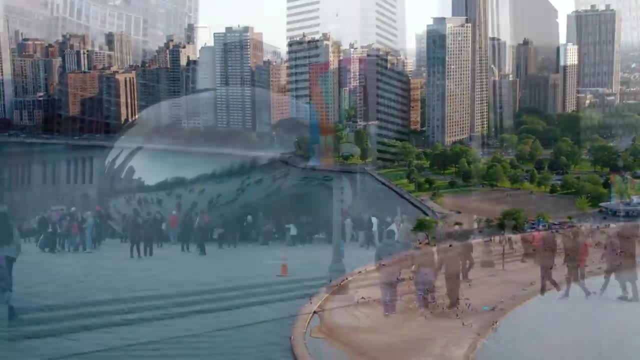 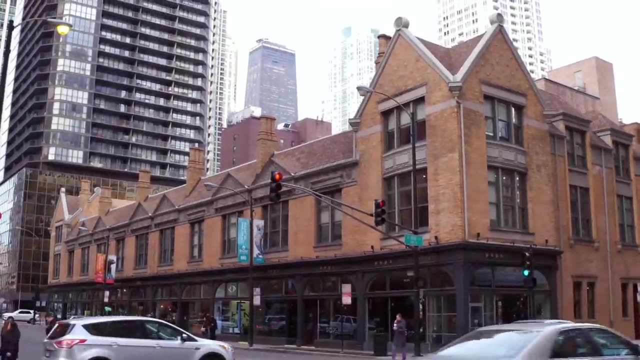 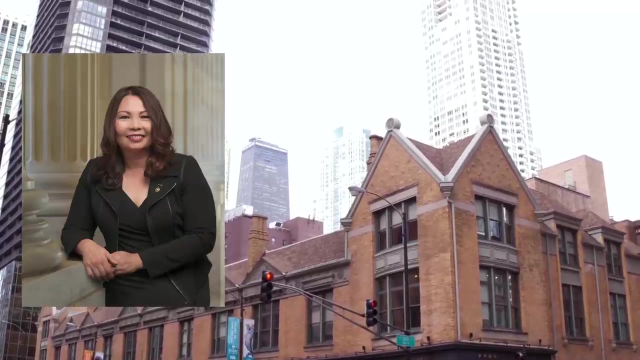 Korean, Pakistani and Japanese. Illinois was the first state to require public schools to teach a unit of Asian American history. They even have an Asian American senator, Tammy Duckworth. She's a combat veteran of the war in Iraq. She served as a US Army helicopter pilot In 2004,. her helicopter was hit by a RPG and obviously crashed and she lost both her legs. She also is the only senator to ever give birth while in office- Not like at her office, It was actually at a hospital, but she was a serving member of Congress at the time. 5.9% of Illinois'. 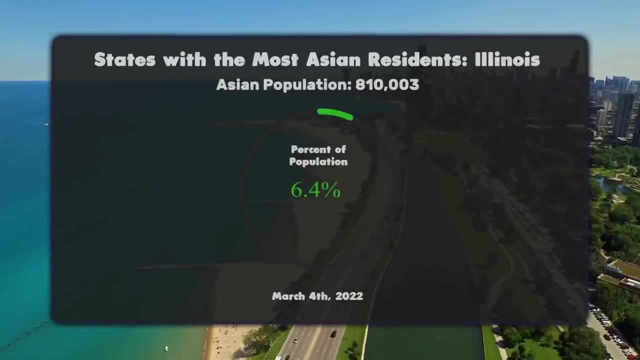 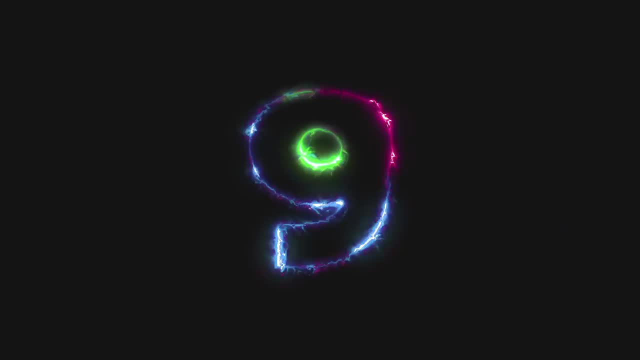 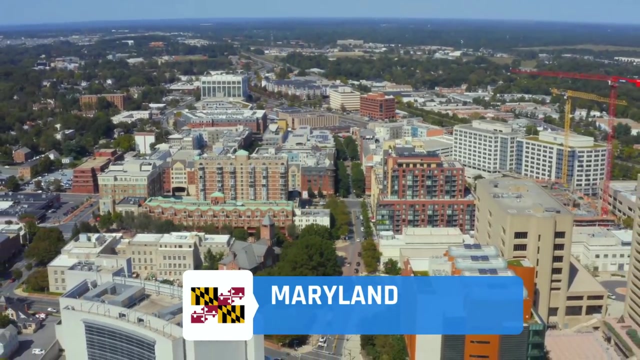 population is Asian. If you go with mixed Asian, that brings them all the way up to 6.45, giving Illinois an Asian population of 810,000.. Number 9, Maryland. Maryland is another state with a very strong Asian population. The 10 largest Asian races in Maryland are Indians, Chinese. 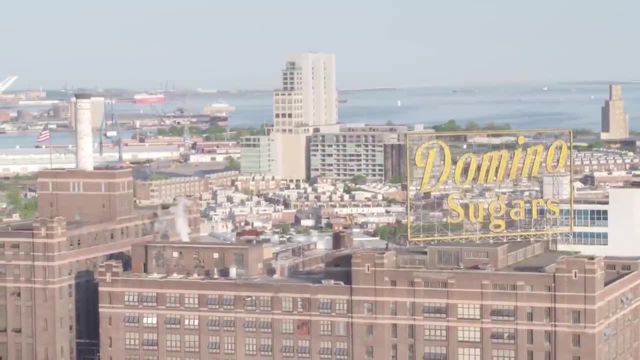 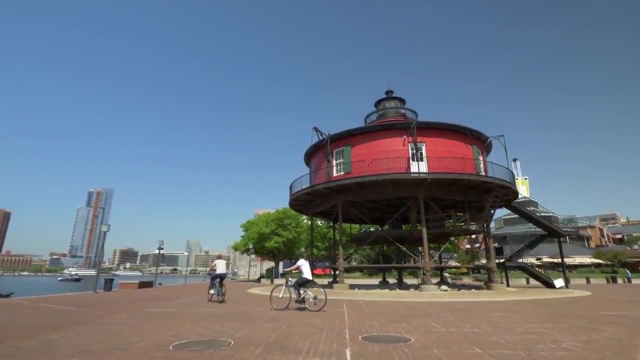 Koreans, Filipinos, Vietnamese, Pakistani, Japanese, Taiwanese, Thai, Burmese. Maryland's first lady Governor Larry Hogan's wife, Yumi Hogan, is a Korean American. She actually makes YouTube videos called Yumi Cooks, where she whips up all. kinds of Korean dishes. I watched a few of them. It's very interesting. The percentage of Maryland's Asian population is 6.9%. When you figure in the mixed Asian population in Maryland you have 7.40%, giving them an Asian population of 451,000 Asian Americans. 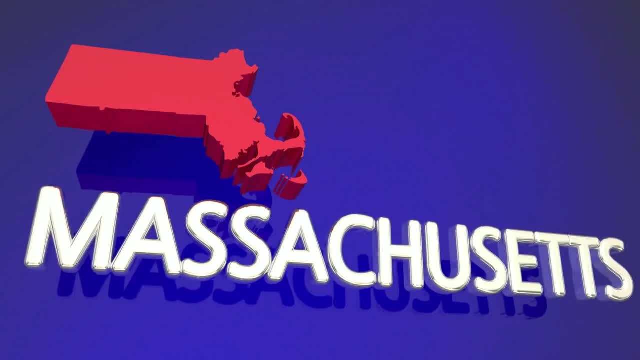 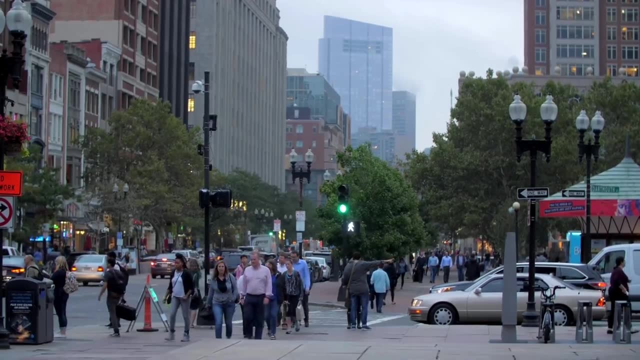 Number 8, Massachusetts. So I have an Asian friend that lives in Massachusetts. He's a Japanese and I Facebooked him and kind of went over the numbers with him. There's like 517,000 Asian residents living in Massachusetts. His thing was: no, I think there's more, but okay. 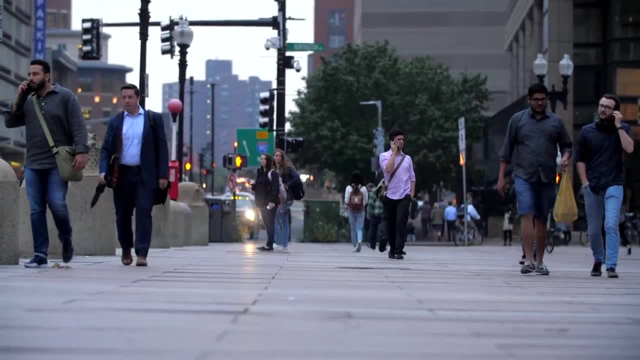 let's say it's 517,000.. Then he goes: did you think it was just me or something, that I sit around and watch Kung Fu Theater and eat chow mein? That's what he told me. I'm like no. 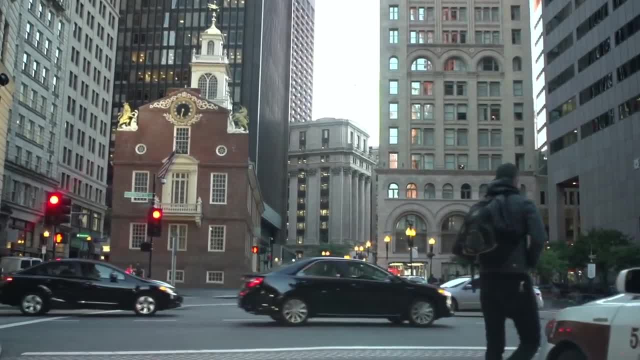 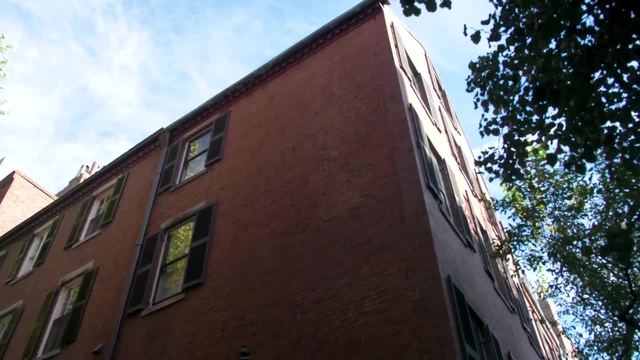 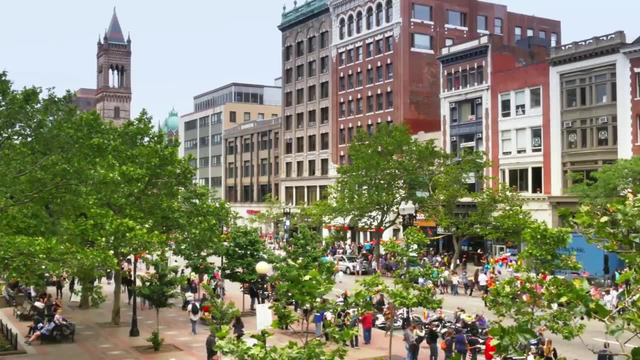 actually speaks four languages: English, Japanese, German and Spanish. He actually worked at one of the embassies for a lot of years. The Asian populations rank like this in Massachusetts: Chinese being number one, followed by Cambodians, Vietnamese, then Koreans. 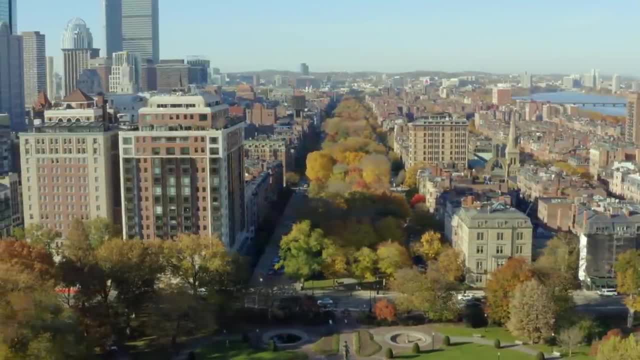 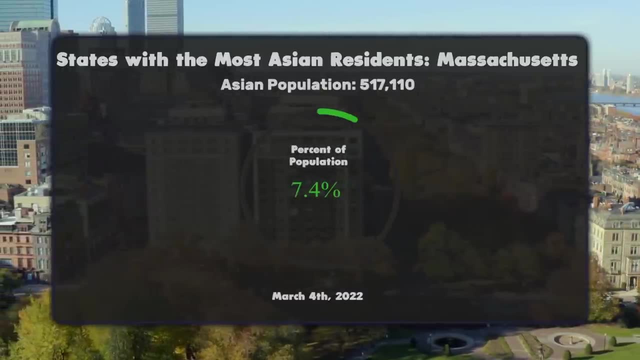 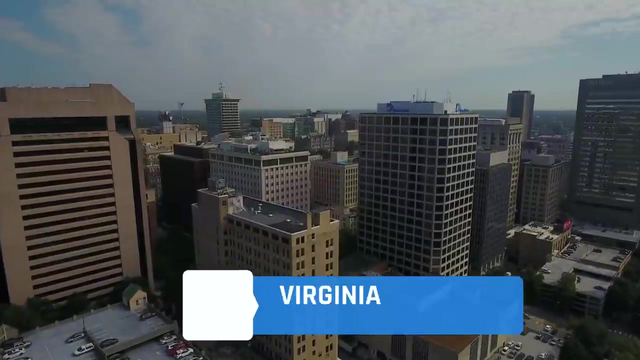 7.2% of Massachusetts population is Asian And if you get into the mixed race Asians it comes up to 7.46, giving them, like I said, about 517,000.. Number seven: Virginia. Virginia is another state with a good size Asian population. that. 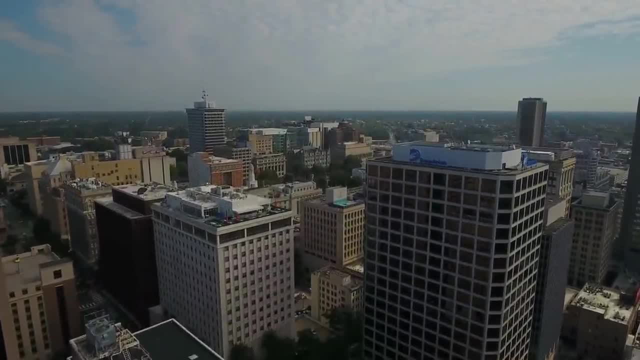 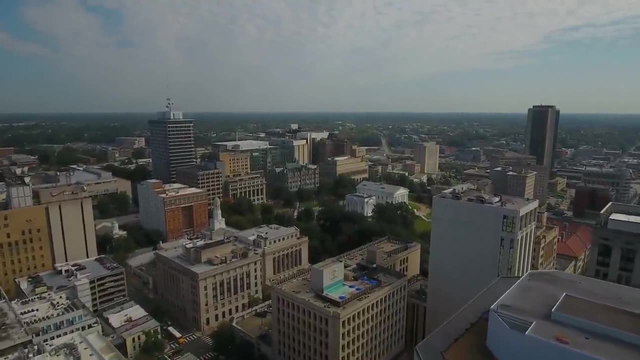 seems to focus in one part of the state And that would be the Northern section with Fairfax, Woodbridge, Manassas, up there near Alexandria and Washington DC. A lot of them will work in government, maybe for other embassies or whatever, but there's a ton of Asian Americans living in. 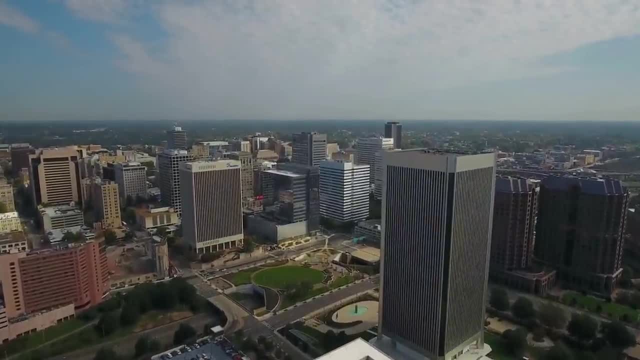 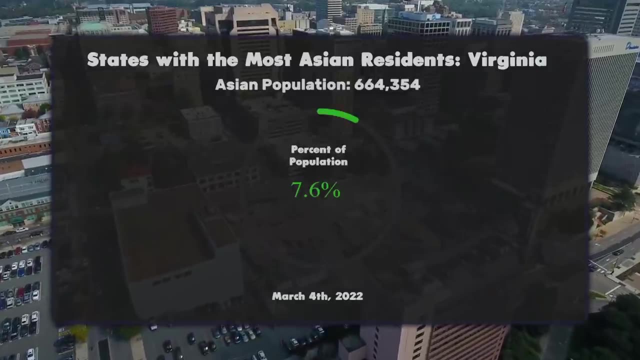 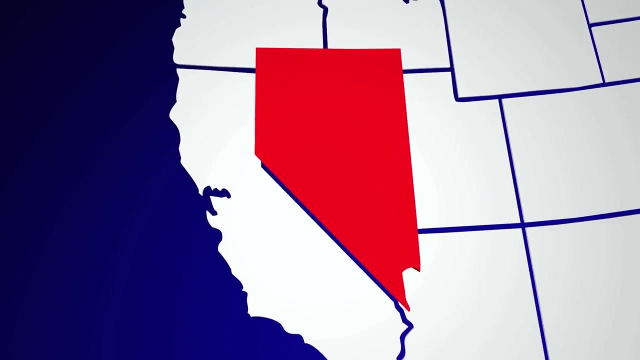 this area. The Asian population of Virginia is 6.9%, But if you count in the mixed race ones it takes them up to 7.69%, Giving Virginia a total Asian population of 664,000.. Number six: Nevada. This one kind of surprised me. I didn't take Nevada as a, you know. 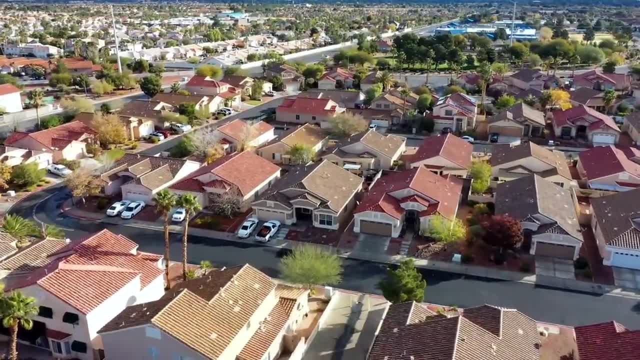 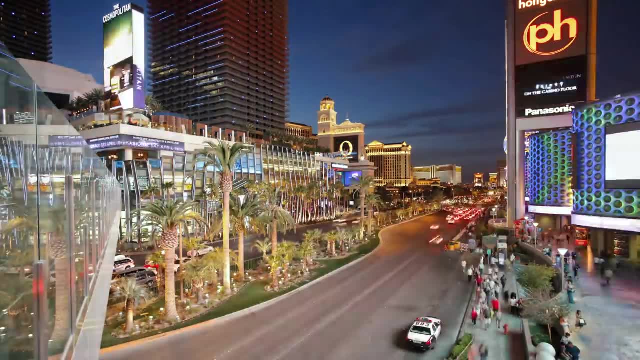 big place for a lot of Asian people. I used to go there a lot. I never really jumped out at me. I know one Asian guy that lives in Nevada. I messaged him. He said: I'm not Asian, I'm actually from Alaska, which of course made me totally uncomfortable. Then, a few minutes later, 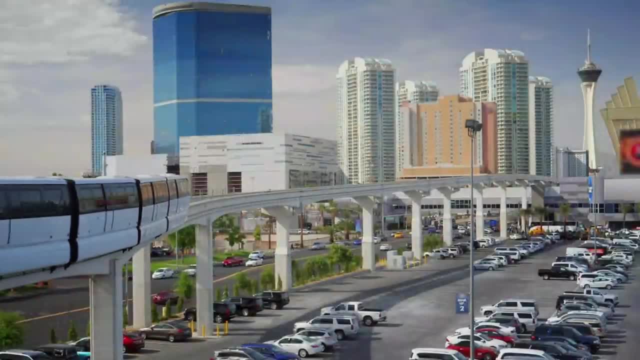 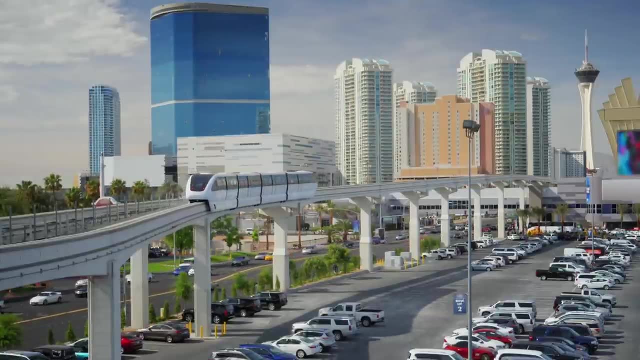 he came back and said: no, he's half Irish, half Korean. So I was like, oh okay. Then I also found out he doesn't live in Nevada, He actually lives here in Oregon someplace- Well, actually Southern Oregon, but he did say when he 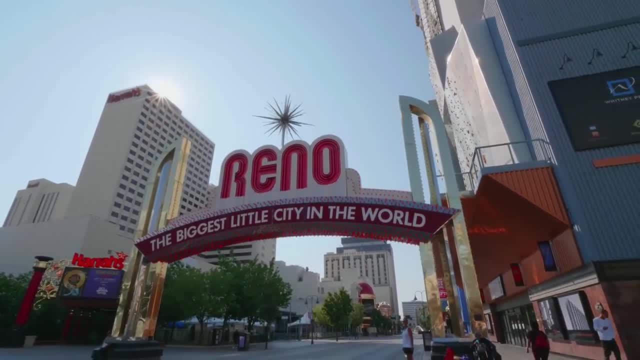 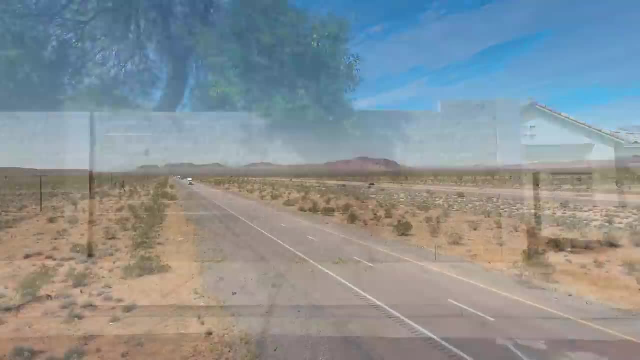 was living in Henderson, Nevada, there was a good size Asian population. He couldn't speak for the rest of the state but he said there's definitely a ton living in the Las Vegas metro area. 8.7% of Nevada's population is Asian. When you figure in the mixed race Asian population in Nevada. 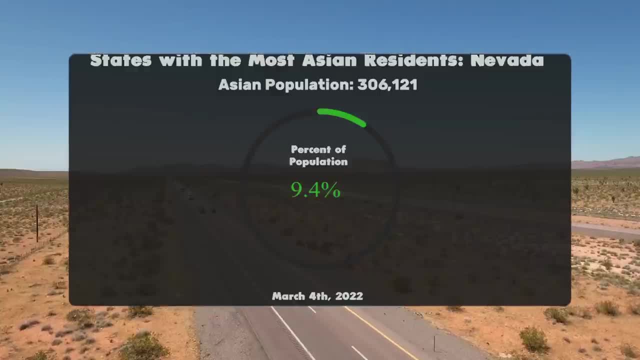 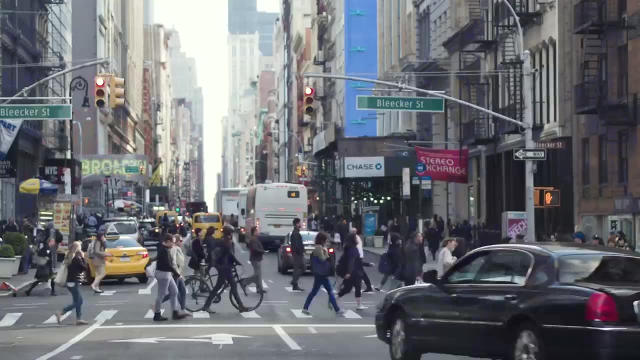 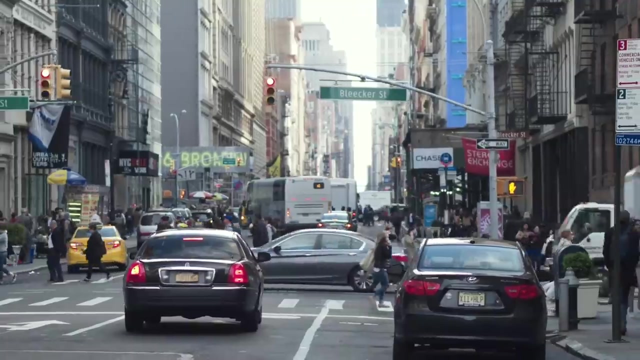 that brings it up to 9.43%, with a total of about 306,000.. Number five: New York. New York has a very large Asian population, Most of it being in New York City. just like most of the population of New York is in New York City, They have some in Buffalo and everywhere else but a. 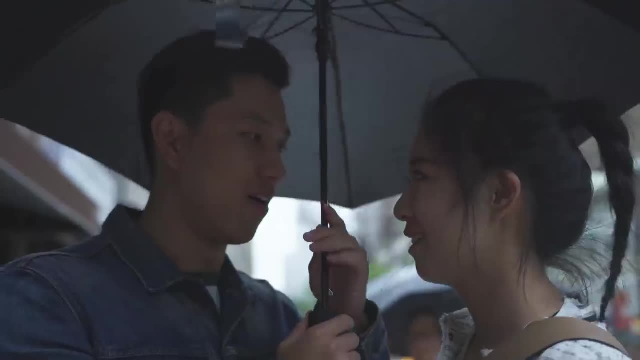 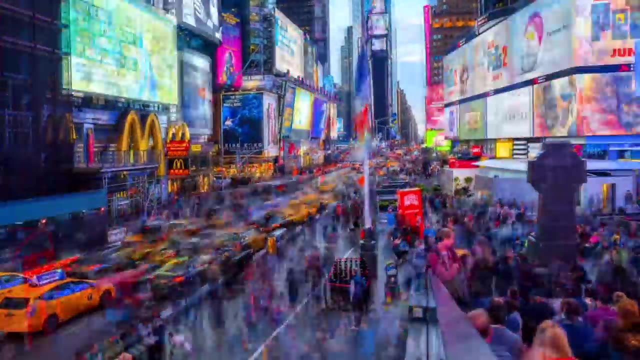 majority of the Asian population lives in New York City and they are Chinese. That's their biggest demographic of the Asian races And in New York City you're going to find the neighborhoods that have the most are Flushing, Lower Manhattan and Bensonhurst alone has about 40,000 Chinese. 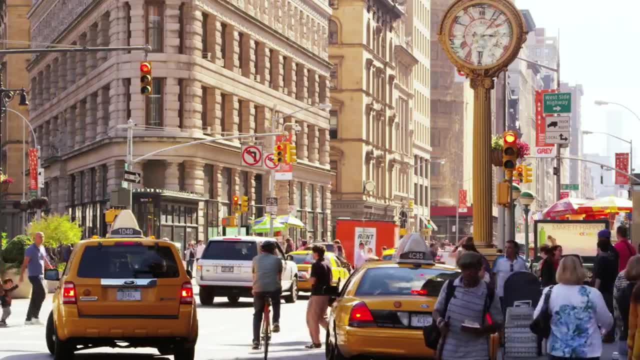 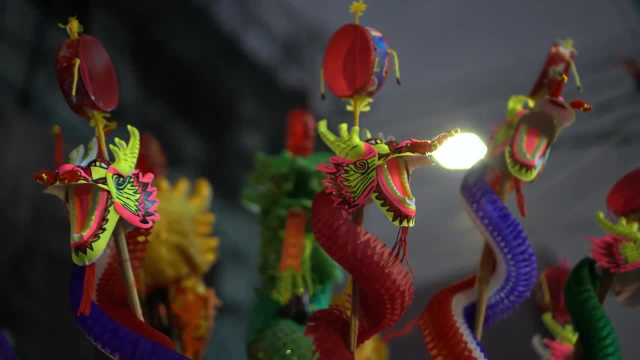 residents, And that's according to the Asian American News Federation. Chinatown in New York City is probably the second best, right behind San Francisco's Chinatown. Well, San Francisco, let's say, in the early 2000s, late nineties. These days, 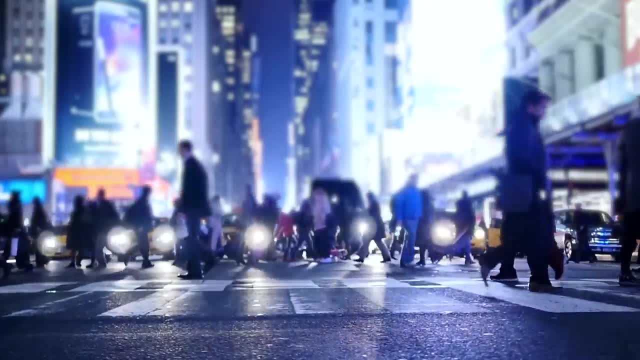 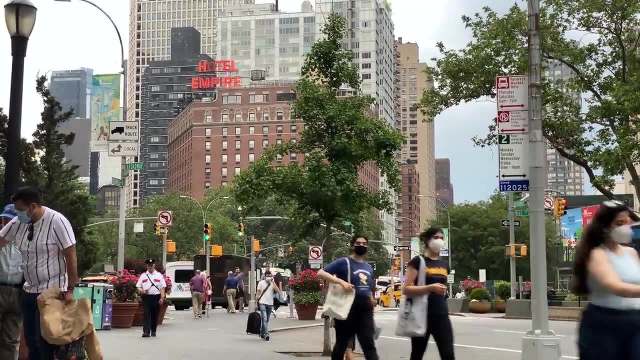 it kind of sucks, But anyway, they have a lot of street vendors and a lot of great places to eat in Chinatown, New York City. I found it strange that the Museum of Chinese in America isn't in Chinatown. It's right outside, on center, in between Grand and Hester, I believe. 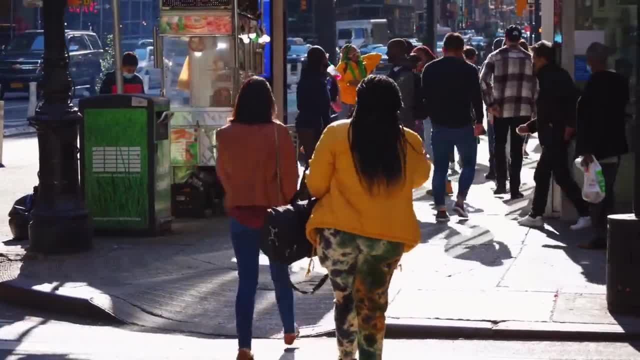 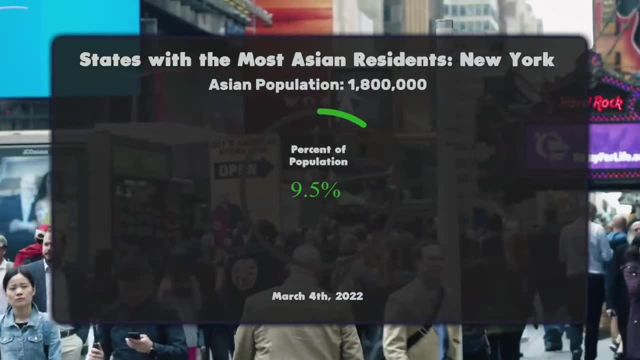 8.9% of New York's population is Asian And when you figure in the mixed race Asian, it comes up to 9.57%, giving New York an Asian population of 1.8 million. Number four: Washington State. If you ever spend any time in Seattle. this one should be no surprise to you. Seattle has been a landing spot for Asian immigrants for generations. For the most part, it is Chinese, Korean and Japanese, with the largest concentration being just outside of Seattle, in Bellevue, Washington. 25% of their population is of Asian descent. 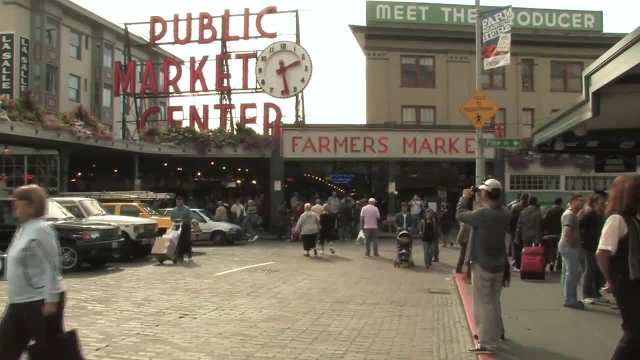 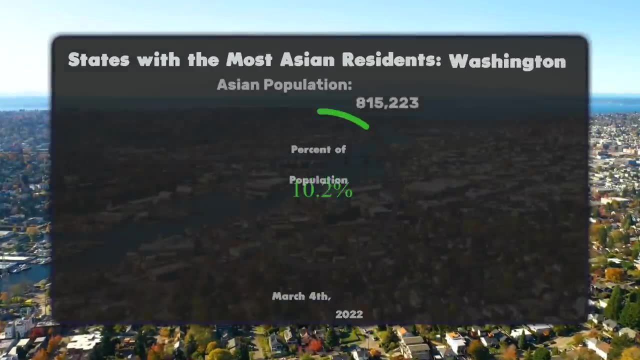 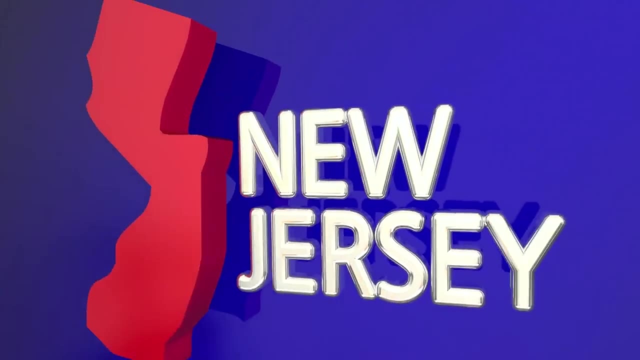 Now the entire state, that's only about 9.6% of the population, is Asian Americans. When you figure in the mixed race, that brings them all the way up to 10.30%, giving Washington State an Asian population of 815,000.. A little bit over Number three, New Jersey, New Jersey's. 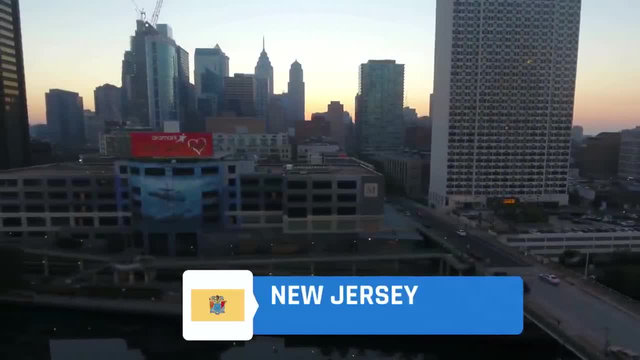 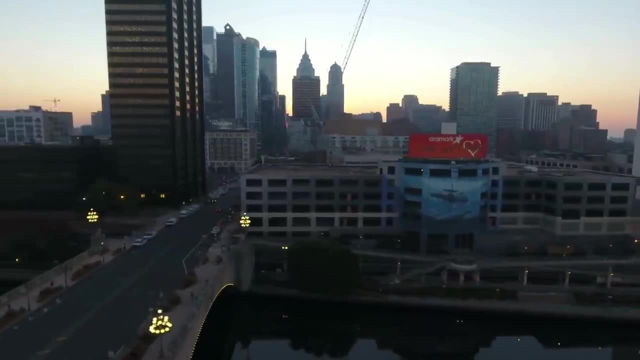 another one of those states. that shouldn't really surprise you. They've got very strong Asian communities here, especially in the Middlesex and Hudson counties. The largest portion of the Asian communities is in New York City, which is the largest Asian community in the state. In fact, it is actually the largest Asian community in the state. The largest Asian community in New Jersey would be Indian, followed by Chinese, Filipino, Korean, Pakistani, Vietnamese and Japanese. And, just like all New Jersey residents, they use the effort far too much and they're just rude, especially in traffic. 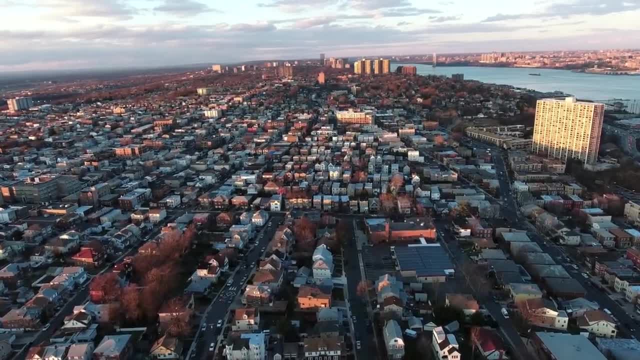 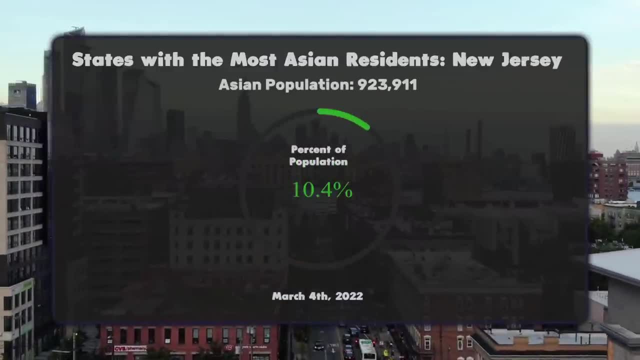 The Asian community accounts for 10% of New Jersey residents, with 10.4% when you factor in the mixed race Asians, giving them a grand total of 923,000 Asians living in the State of New Jersey. Number five: Miami. Well, that's a big one. In the mid to upper 50s Miami maybe would be a big one. Number five: Miami. Well, that's a big one. In the mid to upper 50s Miami maybe would be a big one. The next two states, New York and Boston, might be one, but that's a pretty small one. 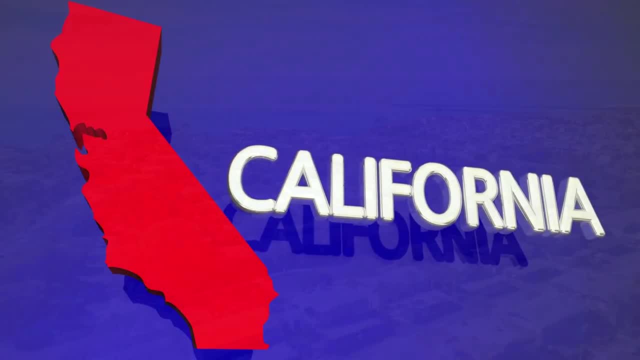 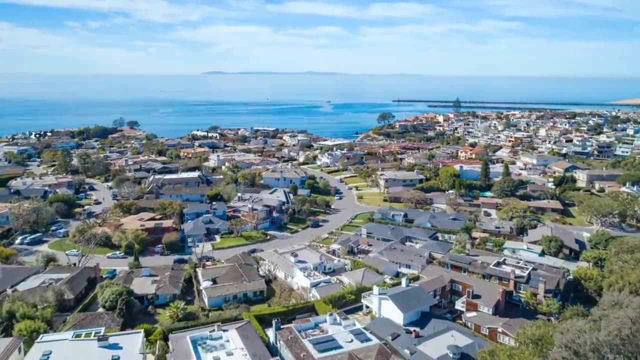 Number two, California. Now the last two on this list are gonna get a little strange because the numbers are so different and that's because of the size of the states. California has a giant Asian community. I grew up in West Torrance, California. Half my friends were Korean or Japanese. Actually, it's more like this: I had a lot of Korean friends that I hung out with on a regular basis. I knew a lot of Japanese people in high school, but they didn't hang out with me. because I was rude and obnoxious, But California has large pockets of Asian communities all over the state. I mean there's a lot of them. Like I said earlier, one of the best Chinatowns in the country is in San Francisco. Actually one of the oldest Chinese restaurants in the United States is in that Chinatown. The oldest continually running Chinese restaurants is in Butte Montana of all places, And it's been family owned the same family. It's like the fourth generation. is running the Pekin Noodle Parlor, But even though California doesn't have the oldest Chinese restaurant, they got some of the best. I've eaten it more than my share over the years. About 15% of California's population is of Asian descent. 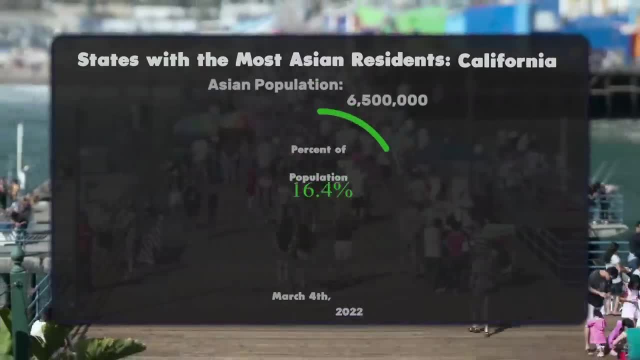 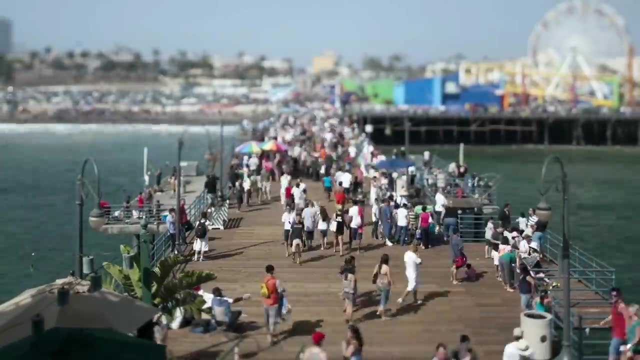 If you figure in the mixed race ones, that is 16.58% of California's population, giving them a total of 6.5 million Asian residents. All right, before we get to number one, don't forget to hit that like button. 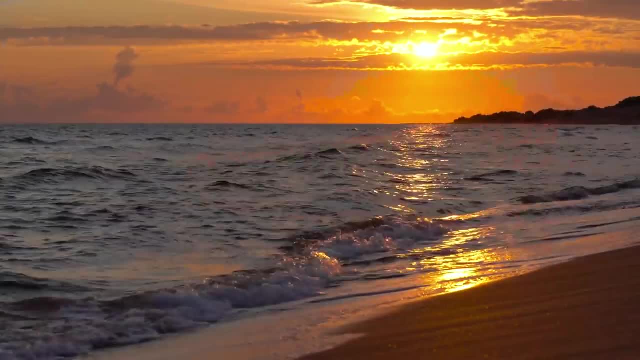 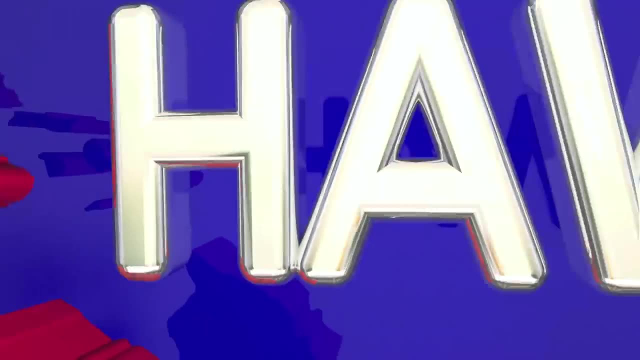 and subscribe if you already haven't. Also, at the end of the video they suggest other videos from this channel to watch. Maybe you could watch one if you got time. All right, on number one And number one Hawaii. This one shouldn't surprise anyone at all. unless you have no clue about what's going on in the world. Hawaii doesn't have near as large of an Asian community as California does. California is like the most populous state we have, So obviously they're gonna have a lot more. So we're focusing on the percentage. and Hawaii blows everyone out of the water when it comes to the percentage, And they also have a giant jump when you go from just Asian to multi-race Asian. 75% of the foreign born population in Hawaii is of Asian descent Back in the 80s and 90s.